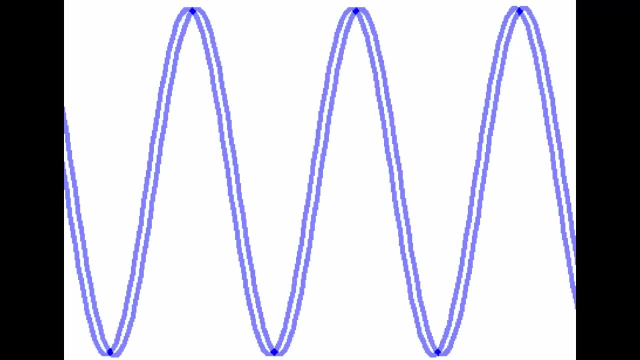 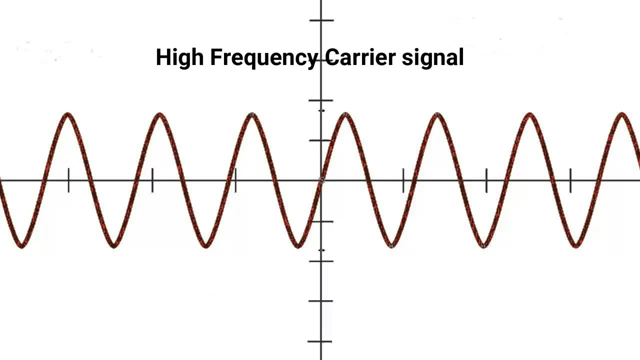 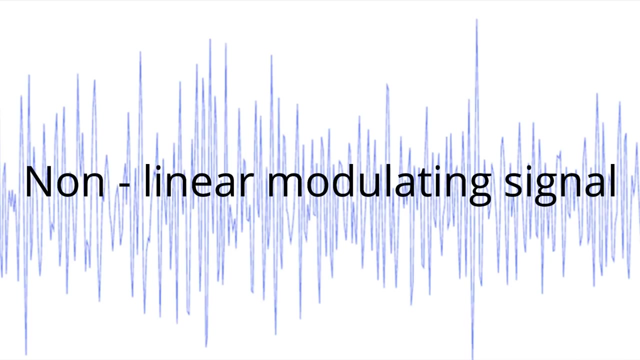 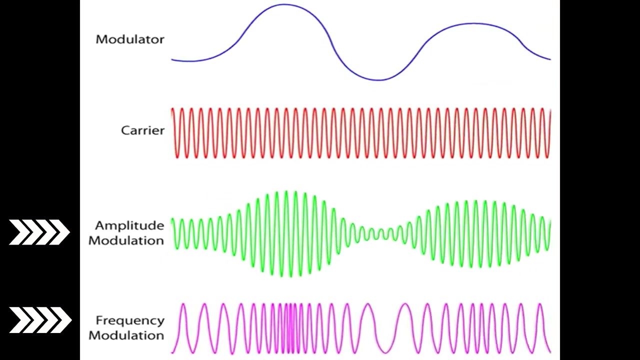 Generally, when we describe a signal, we talk about its 3 important characteristics: Frequency, amplitude and phase. Modulation is a simple process in which a carrier signal of constant phase, frequency and amplitude is modified by non-linear input signal. As a result, we will have a signal output which changes its characteristics corresponding. 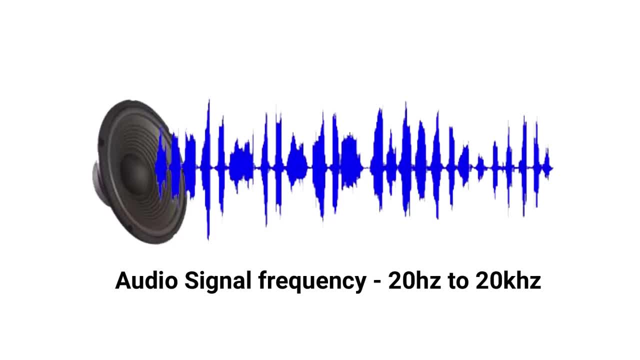 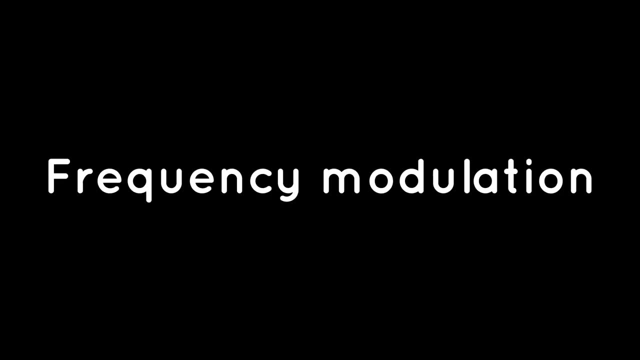 with modulating signal. In most wireless communication systems, audio signal of frequency ranging from 20 Hertz to 20 kilohertz will be used as modulating signal. now let's take a look at the three basic types of modulation: frequency modulation in this type of modulation. frequency of the carrier. 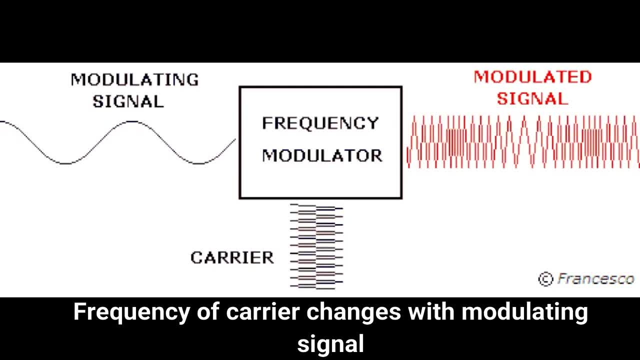 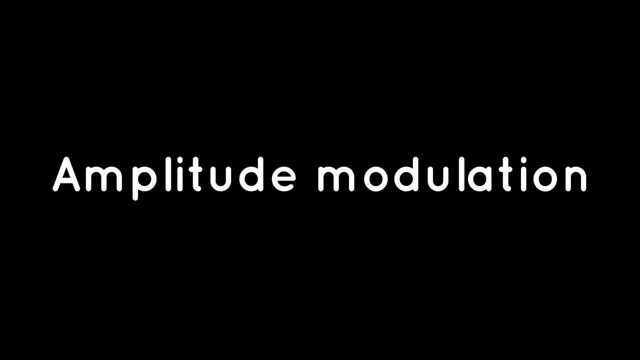 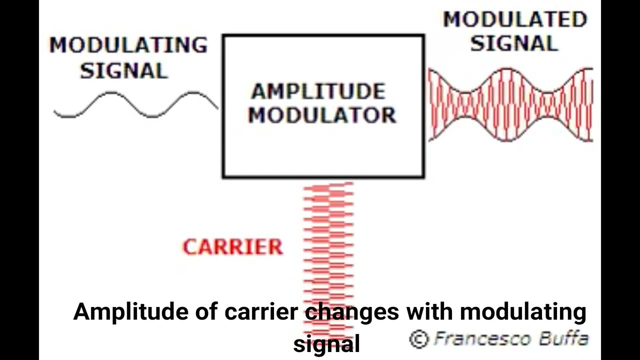 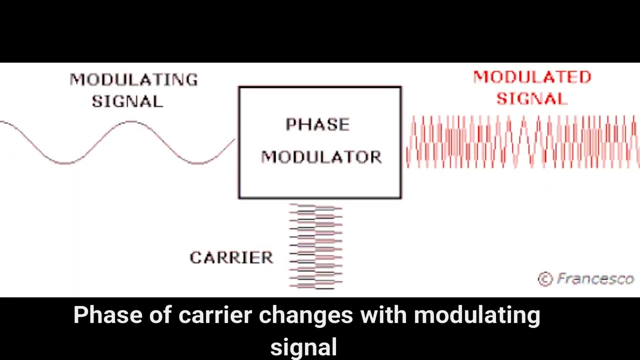 signal will be altered with respect to modulating signal. as a result, we will obtain modified frequency signal in output amplitude modulation. here amplitude of carrier signal will be altered with respect to modulating signal and we will get amplitude modified signal as output phase. modulation phase of the carrier signal will be modified in this method and we 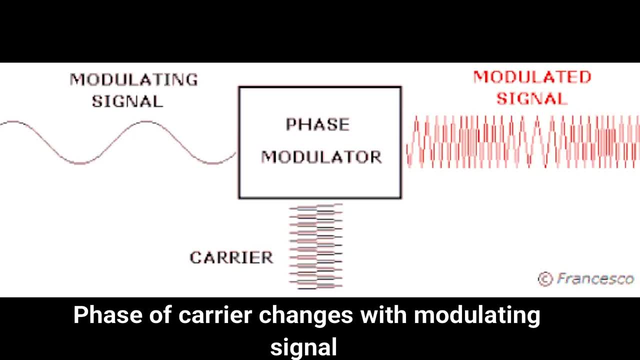 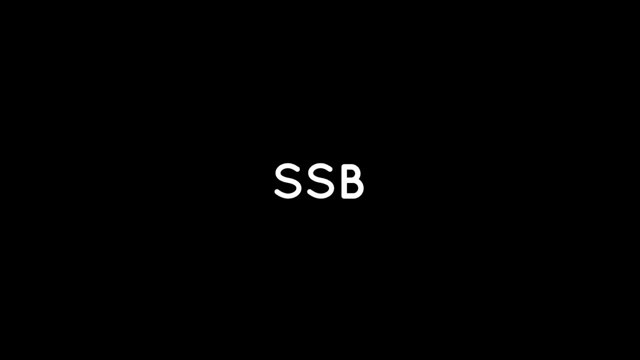 will obtain phase modified signal in the output. apart from these three, there are many other modulation techniques like DSP, SSB, VSB, QAM, ASK and a few more: FSK, PSK and much more. Let's take a look at the three main advantages of modulation. 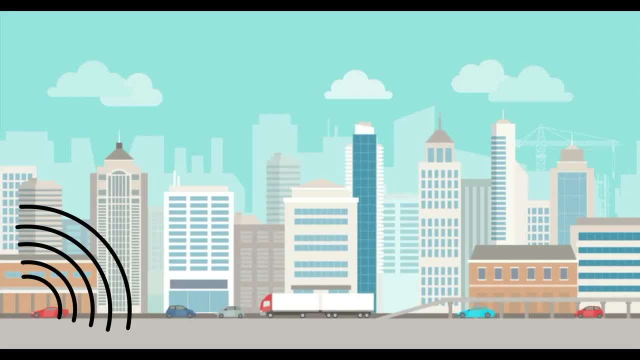 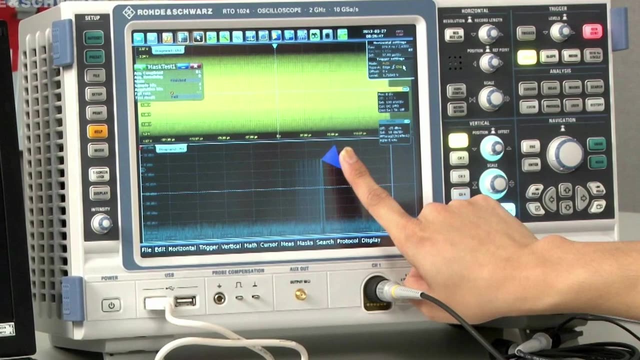 Number 1. To transmit the signal to long distances. Low frequency signals like audio or any other signals are incapable of propagating to long distance on their own. When modulating them with a high frequency carrier signal, the modulated output will obtain high frequency characteristics and, as a result, it can propagate longer and in. 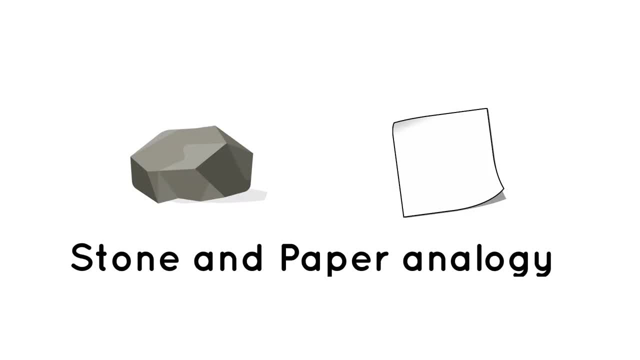 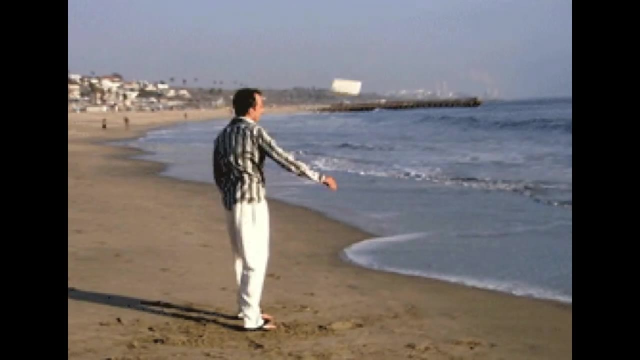 turn, provides more range to the user. This can be simply explained using famous tone and paper analogy. Imagine a paper as your audio signal, and when you throw it in the air, it's so obvious that paper will not go any distance, since it lacks the weight.